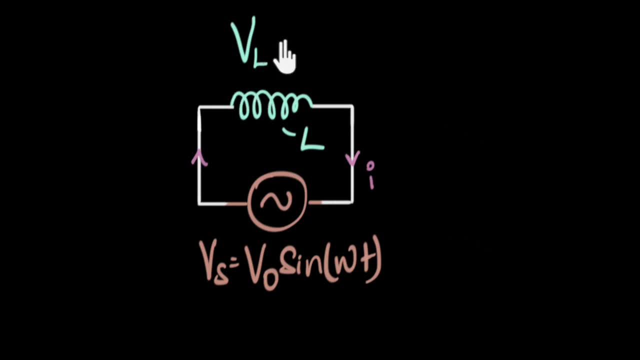 that the magnitude of that voltage, which I'm just gonna call as VL, that will always equal L times, di over dt, Di over dt. And this expression is basically saying that you know changes in current and the quicker the current tries to change, the larger emf or the larger 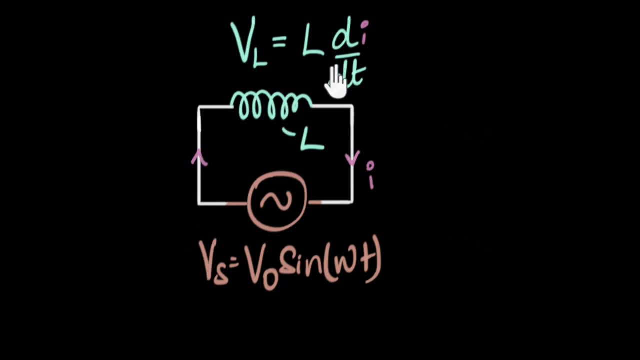 voltage it induces and, of course, if you need a refresher or more clarity on where this comes from, we've talked a lot about that in our previous videos on inductors. feel free to go back and check that out. but now let's see if we can use this to build our equation. so the next immediate 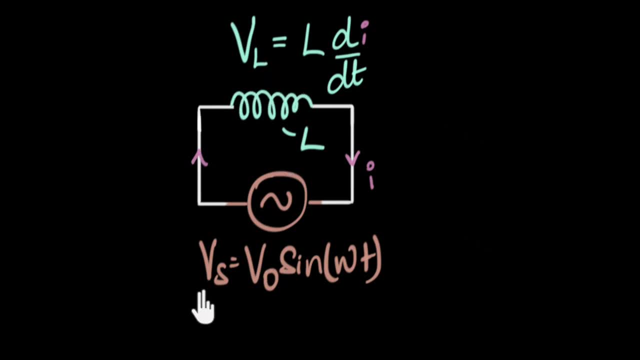 question i have is: what direction is this voltage compared to our source voltage of the generator? so for that, let's say our source voltage is continuously fluctuating. at one point this will be higher, at higher voltage, and then this will be at a higher voltage and this will be our hydro. 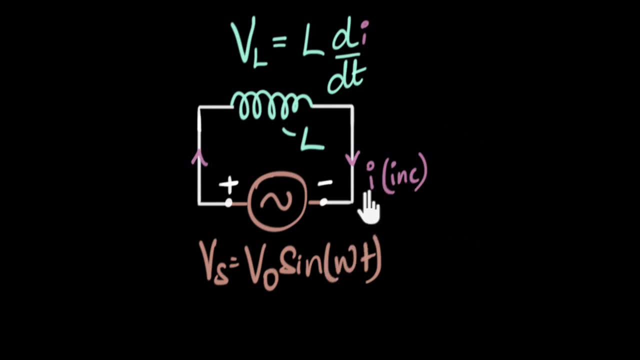 is increasing actually, and therefore, because the current is increasing, our inductor says: uh-uh, i hate changes in current, i'm going to try and decrease the current. okay, because it wants to decrease the current, it's going to try and push back the current and to do that, it puts a high. 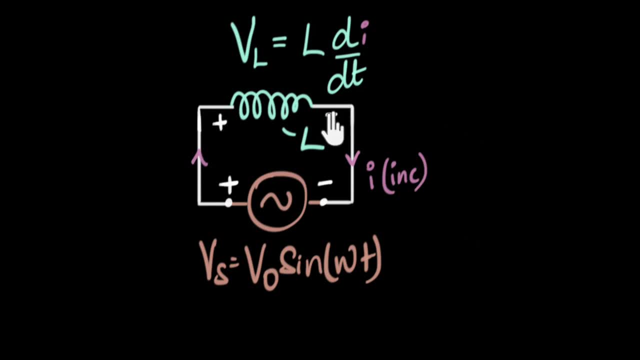 voltage on this side and a low voltage on this side, and so this is the polarity of that induced voltage, and you can immediately see that the polarity of the source voltage and the induced voltage is exactly the same, and because there are no circuit elements in between, we know that. 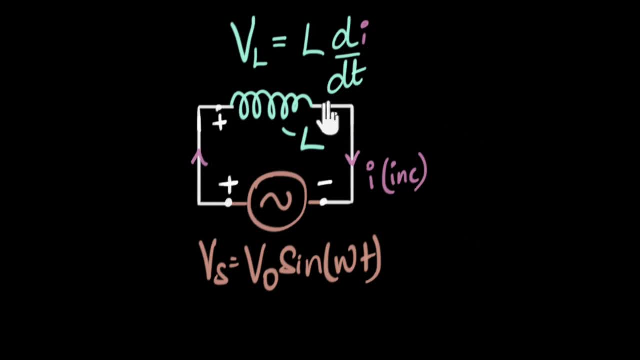 this voltage in this point and this point is at the same potential. this point and this point is at the same potential. in other words, this voltage should exactly equal this voltage, both in magnitude and direction, and so i can use that to figure out what the current is. so let me go and write that. 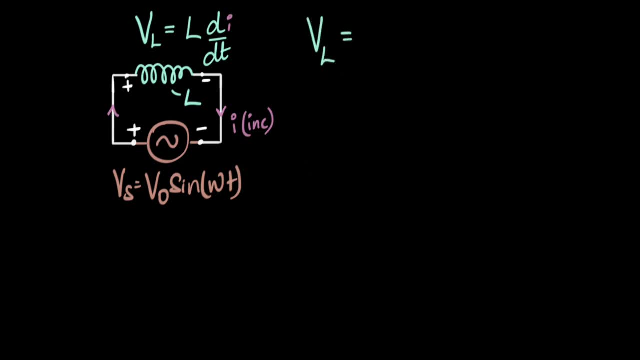 so the voltage across the inductor should exactly equal the source voltage or the generator voltage, both in magnitude and direction. and so if i substitute i get vl equals l, d, i over dt, so d of dt over i. and at this point one confusion i always had is if we go back- and you know we go back to inductors, we said that the emf 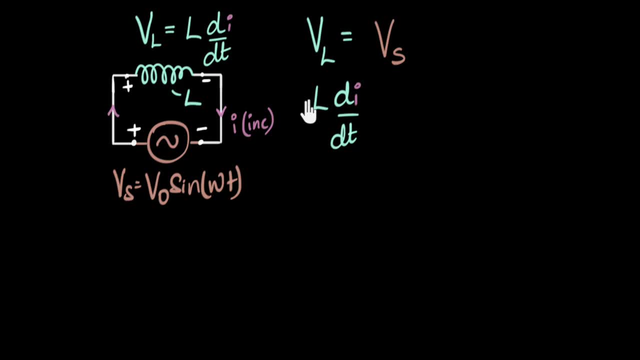 induces negative ldi over dt. so should i put a negative sign over here? well, remember, the negative sign is only telling us the direction of the voltage. it's saying it's in the opposite direction of the change in the current and over here. we've already included the direction over here, including: 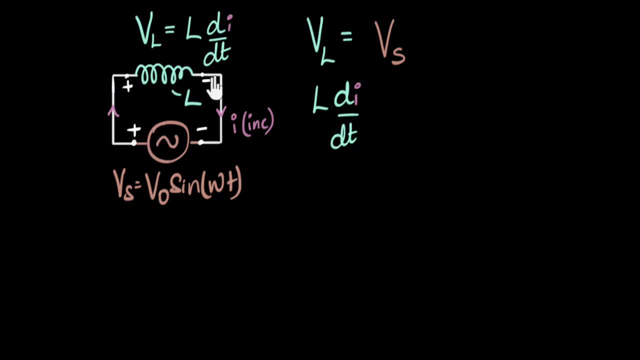 the direction we're. we realized that they both have the same polarity right, so we've already taken care of the direction, so you don't have to worry about the negative sign. and that equals v naught sine omega t. and now we see an equation which is not just an algebraic equation, it's a differential equation. 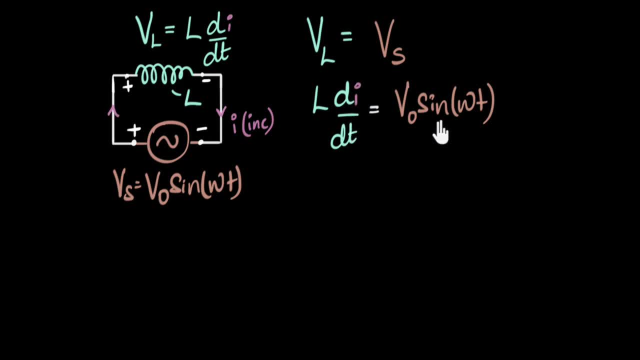 which basically means there is a differentiation term over here, and some differential equations can be very tricky. this turns out to be one of the easier ones, because to solve this all we have to do is separate all the i terms and all the t terms on one side, so we have a differential equation. 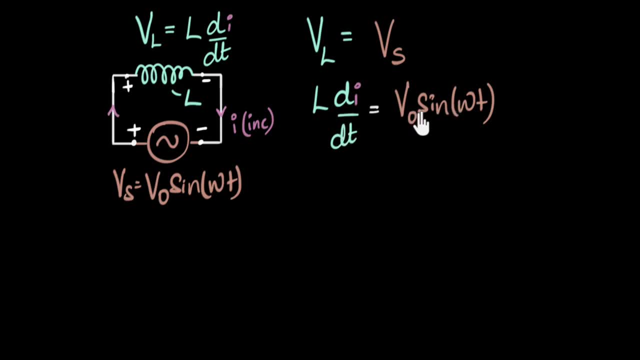 so we can separate them on two different sides and then we can just integrate. now it'll be a great idea to pause the video and see if you can integrate this yourself and see what the expression for current is going to be all right. so i'm going to rearrange, just to have di on one side. 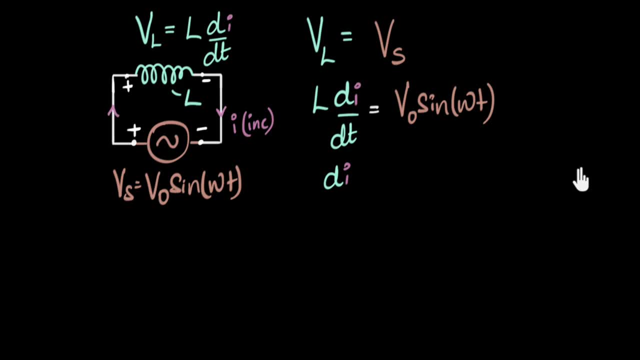 so left side will only put di and so on the right hand side i will get, if i just rearrange, i'll get v naught sine omega t. i'll get a dt over here and i'll get divided by l. and now, because i've got the i terms and the t terms, i can integrate. and if i integrate, integral of di is just i. 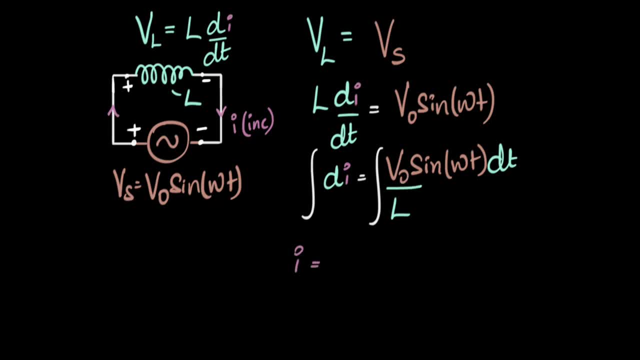 and that equals v naught over. l is a constant. i can pull that outside the integral. and what's the integral of sine omega t, dt? well, that integral, i'll directly write the integral over there. that's going to be minus cos omega t divided by omega, and whenever we integrate, there's going to be a. 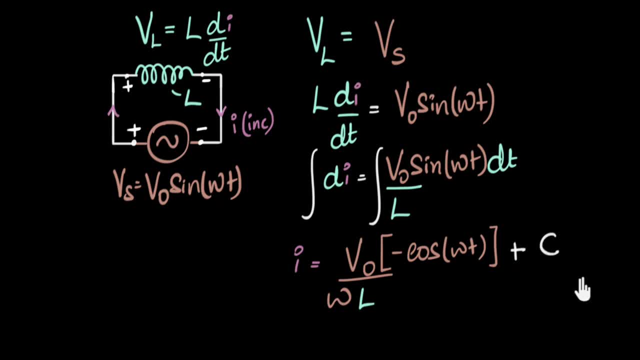 constant. we need to put that constant, and there we go. so this is our expression for the current, and you can immediately see that this is something that we don't know. if you can figure out what the value of that constant is, we are done. so how do we figure this constant out? first of all, what does it? 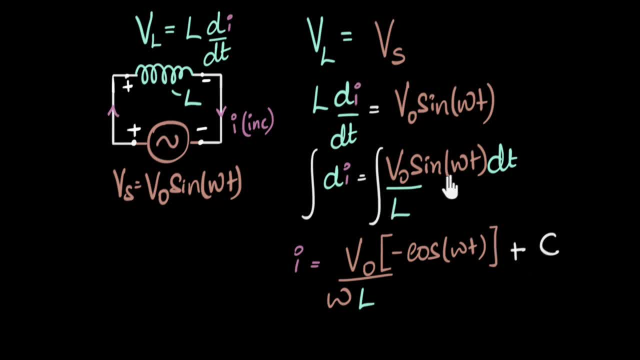 even mean. but remember, integrals is basically like integration is like doing reverse of differentiation, asking what function should i differentiate to get this as the answer? so if you actually take this and differentiate and you can try that, you will actually get this number. differentiation of negative sign: so the negative cancels out and the omega pops out and that cancels with this. 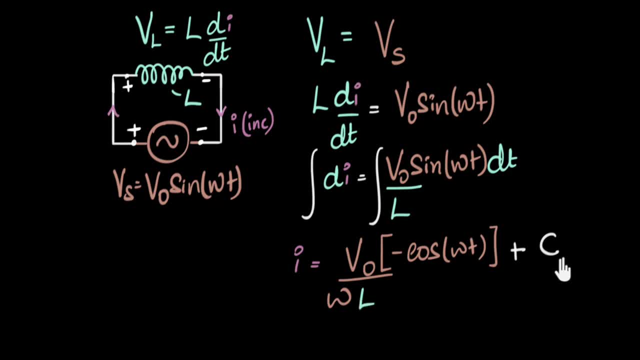 however, remember, differentiation of constant is a zero, which means i can also differentiate this plus hundred, or i can differentiate this plus thousand, and then all of those numbers will still give me this value, and so the integral is saying: i don't know what this constant is. that's, that's. 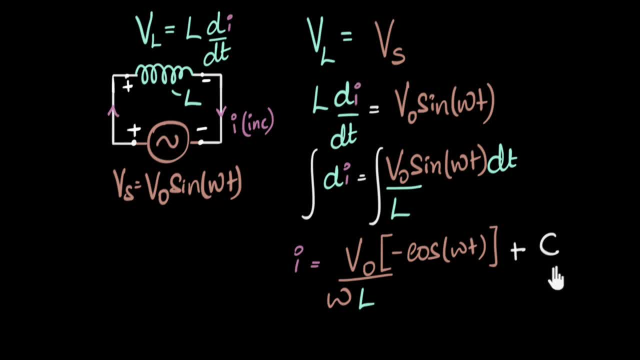 your job, mahesh. it's your job to figure the value of the constant out. so now my question is: how do we figure this out? maths is not going to answer that. we need physics, and one of the powerful ways of figuring out values of constants- whenever i give an equation- is we say hey, it's a. 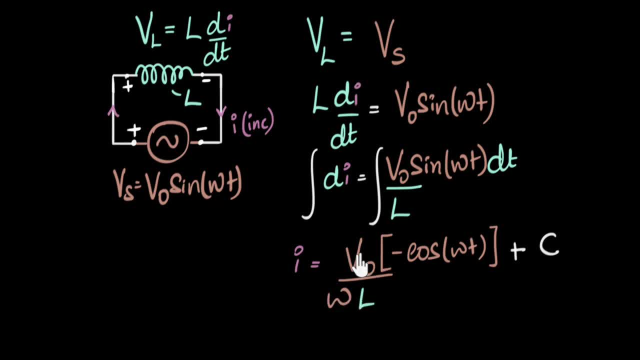 constant, which means it does not depend on the values of voltage or v naught, or does not depend on the values of omega or l. so we can put whatever values of v naught, you know, omega, whatever values we want, and then see if we can figure out what the value of c is going to be. it's a very powerful. 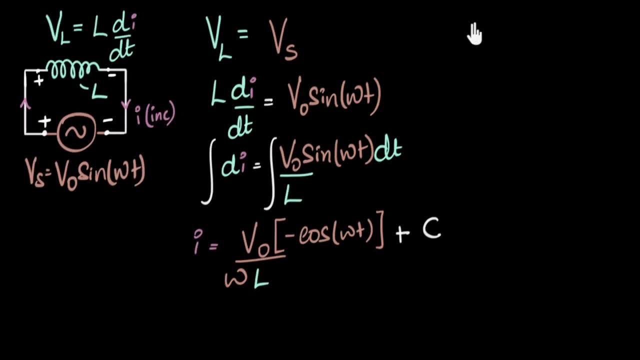 method. let me show you what i like to do over here. let's say, in this particular example we put the v naught value to be zero. if this is zero, that means our source voltage is going to be zero. so if we put the v naught value to be zero, then the current is always going to be zero. so i'm basically saying: 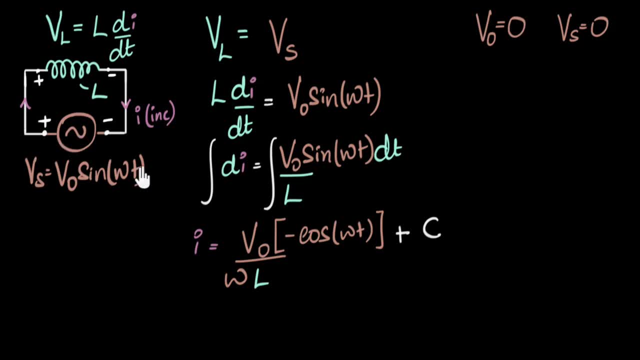 i'm basically saying i'm not going to put any generator in this circuit, okay, and i want to know what the current is going to be based on this equation. so, from this equation, current is going to be: well, this part will be zero, because v naught is zero, but there is a constant. so, according to,